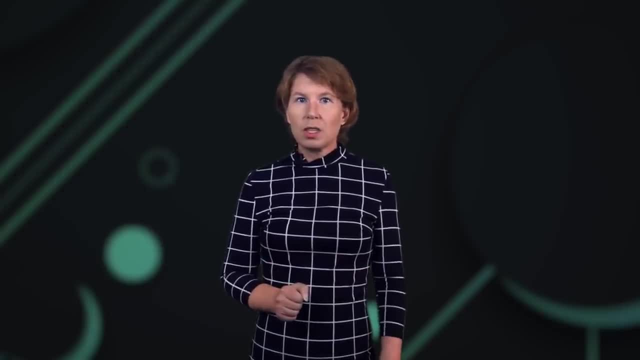 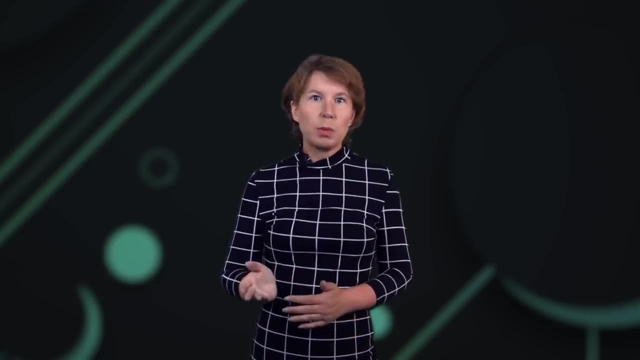 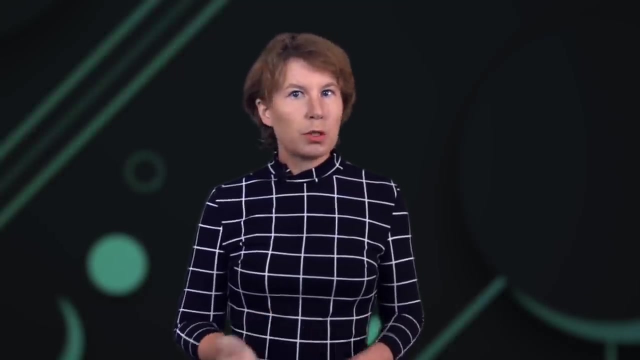 if that's a notion of reality you don't want to use, that's totally okay, but then I challenge you to come up with a different notion that is consistent and agrees with how most people actually use the word. Interestingly enough, not all numbers are real. The example I just gave was for integers. 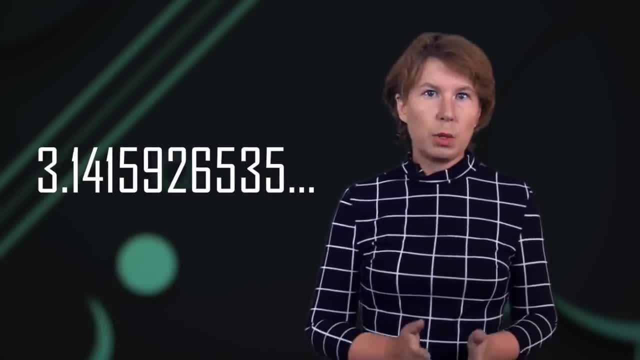 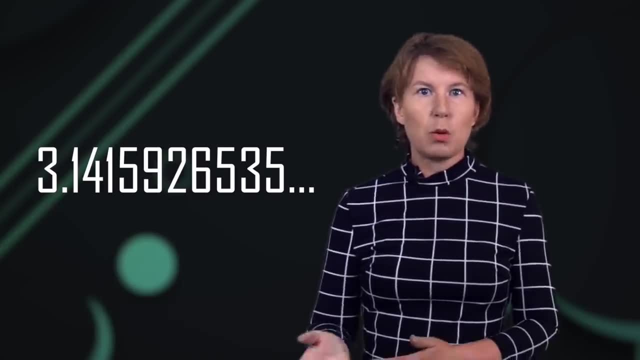 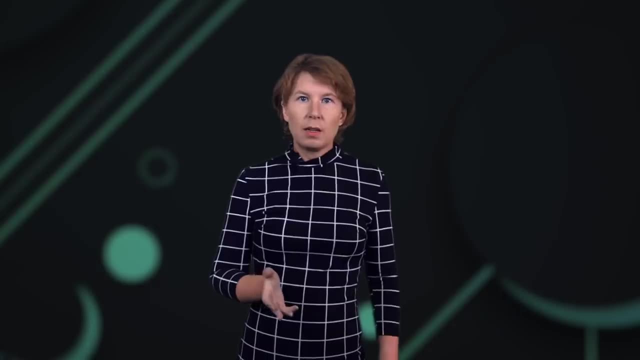 But if you look at all numbers with infinitely many digits after the decimal point, we don't actually need all those digits to describe observations, because we cannot measure anything with infinite accuracy. In reality, we only ever need a finite number of digits. Now, 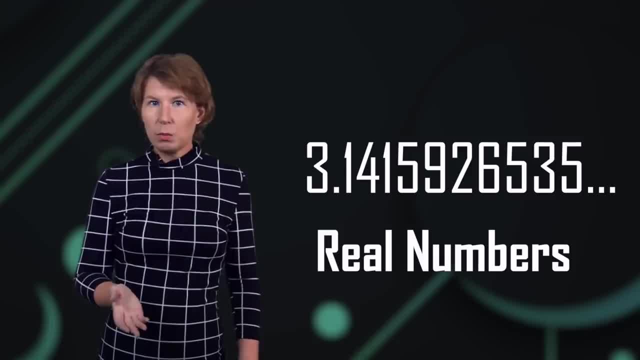 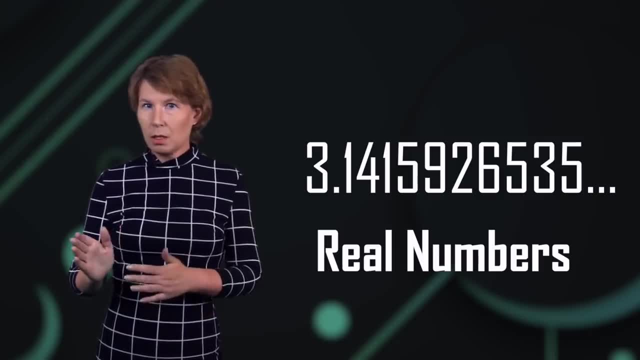 all these numbers with infinitely many digits are called the real numbers, Which means odd as it may sound. we don't know whether the real numbers are real, But of course physics is more difficult than just numbers. For all we currently know everything. 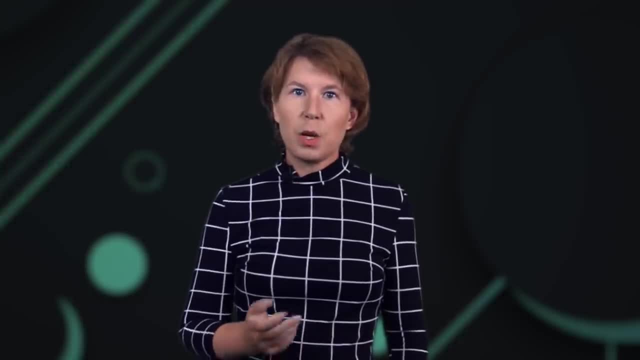 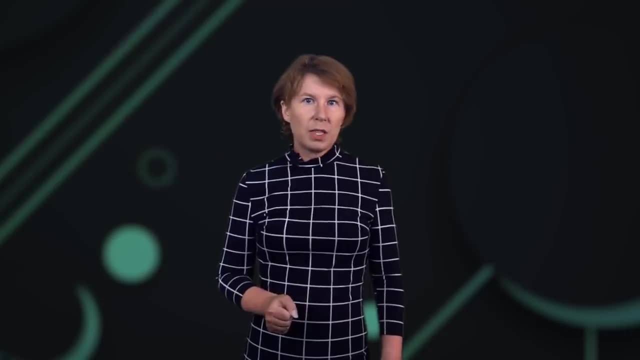 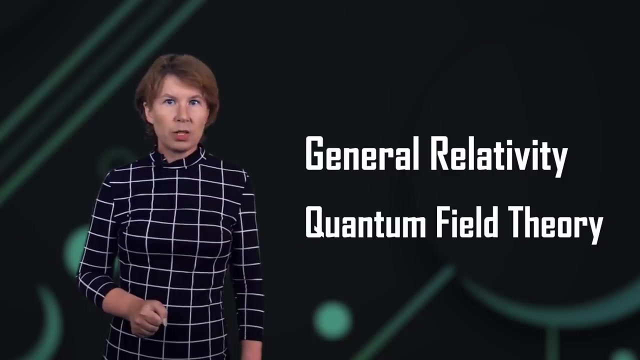 in the universe is made of 25 particles held together by four fundamental forces: gravity, the electromagnetic force and the strong and weak nuclear force. Those particles and their forces can be mathematically described by Einstein's theory of general relativity and field theory, theories which have been remarkably successful in explaining what 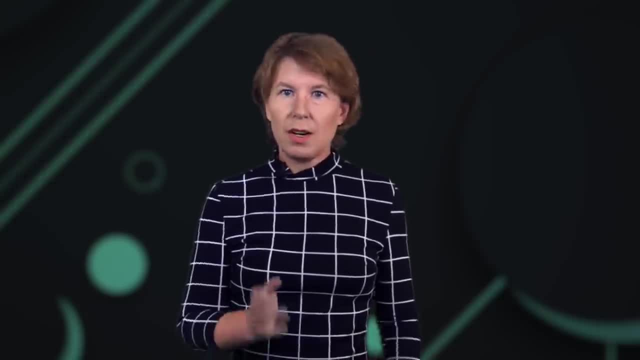 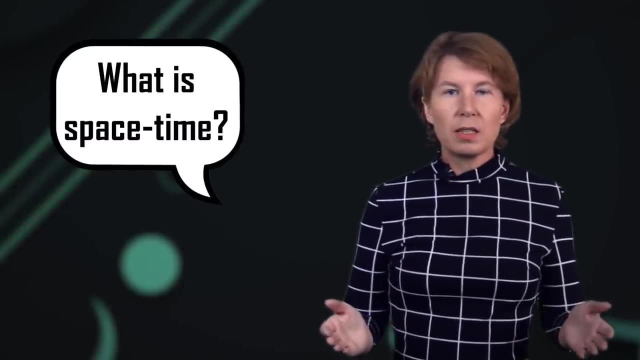 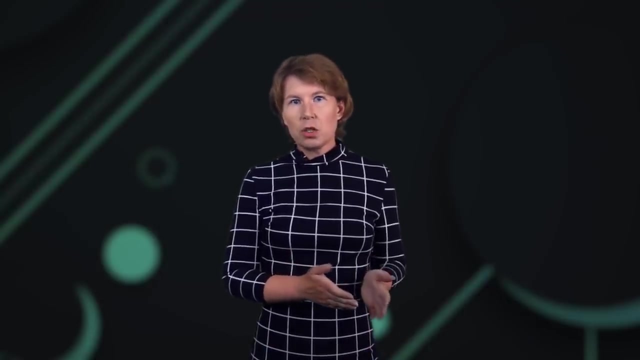 we observe. For what the science is concerned, I'd say that's it, But people often ask me things like what is space-time, What is a particle? And I don't know what to do with questions like this. Space-time is a mathematical structure that we use in our theories. This mathematical structure is defined by its properties. Space-time is a differentiable manifold with Lorentzian signature. it has a distance measure, it has curvature and so on. It's a math thing. We call it real because it correctly describes our observations. 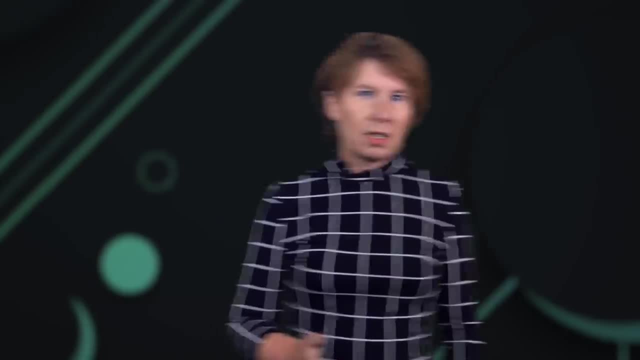 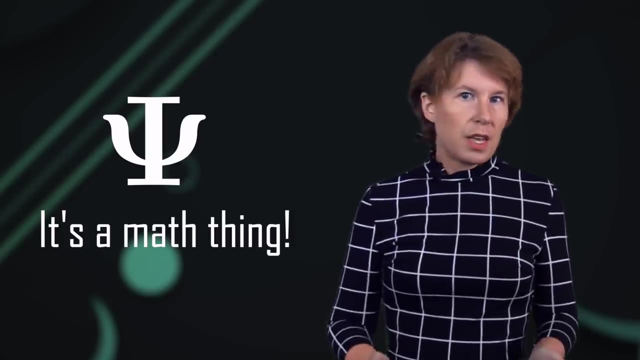 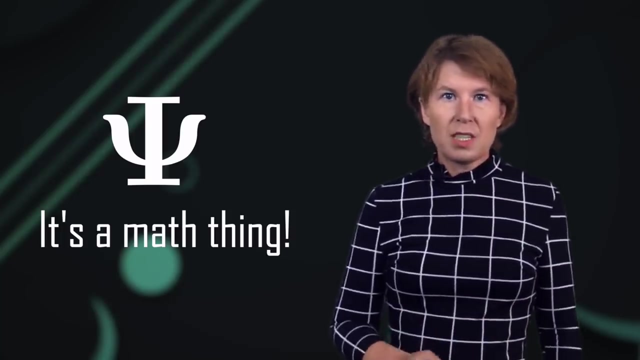 It's a similar story for the particles. A particle is a vector in a Hilbert space that transforms under certain irreducible representations of the gauge groups. That's the best answer we have to the question what a particle is. Then we call those particles real because they correctly describe what we observe. 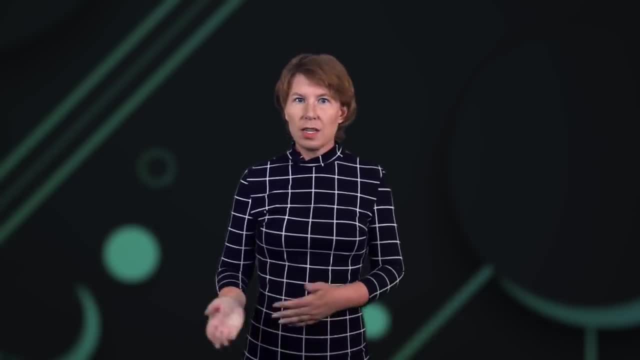 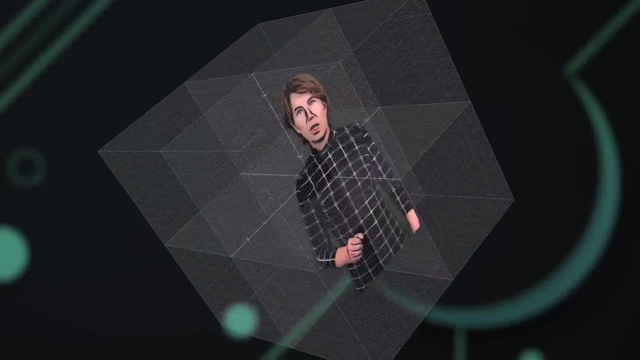 So when physicists say that space-time is real or the Higgs boson is real, they mean that a certain mathematical structure correctly describes observations. But many people seem to find this unsatisfactory. Now, that may partly be because they're looking for a 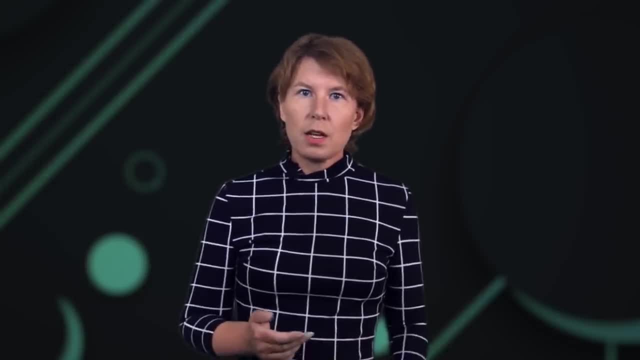 simple answer and there just isn't one. But I think there's another reason: It's that they intuitively think there must be a reason, And that's because they're looking for a simple answer and there just isn't one. But I think there's another reason: It's that they intuitively think there must. 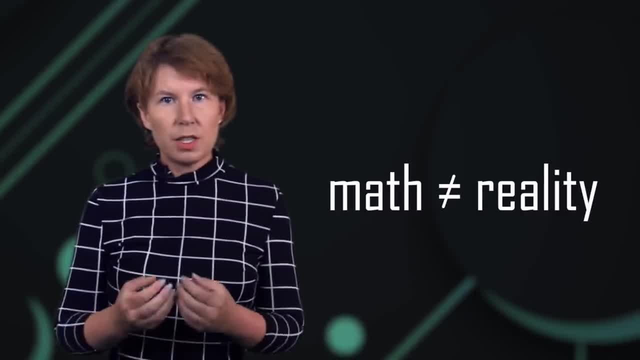 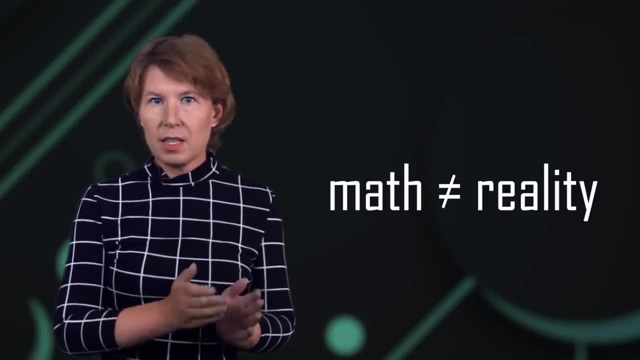 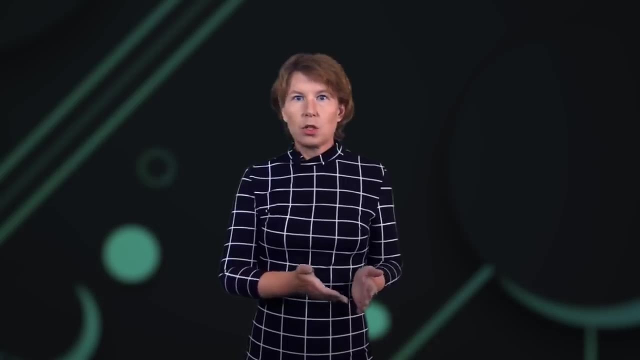 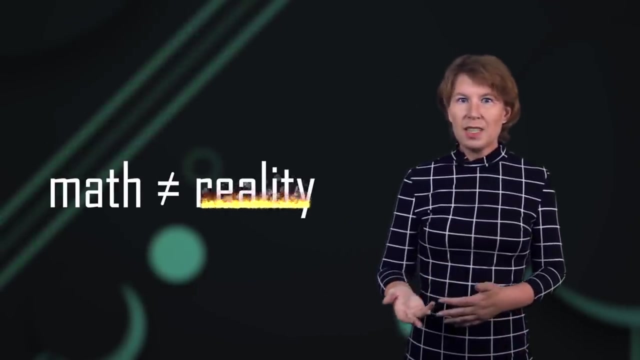 be something more to space-time and matter, something that distinguishes the math from the physics, Something that makes the math real or, as Stephen Hawking put it, breathes fire into the equations. But those mathematical structures in our theories already describe all our observations. This means just going by the evidence. you don't need anything. 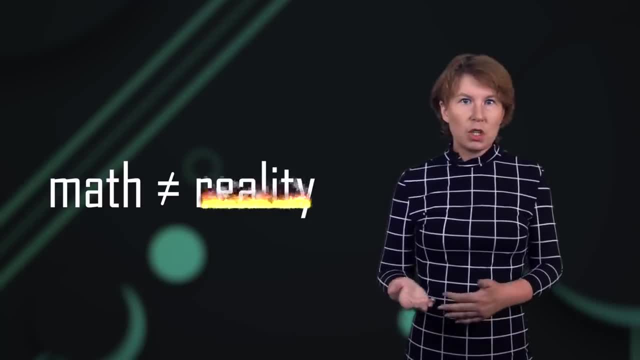 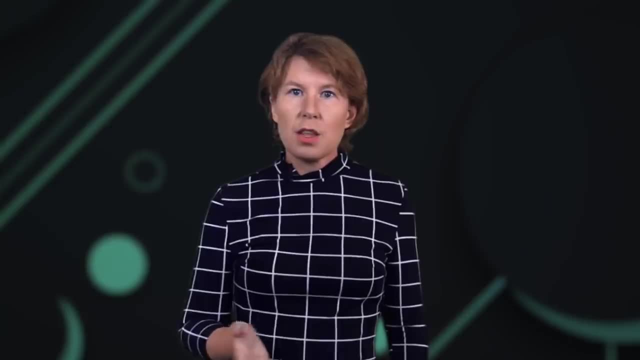 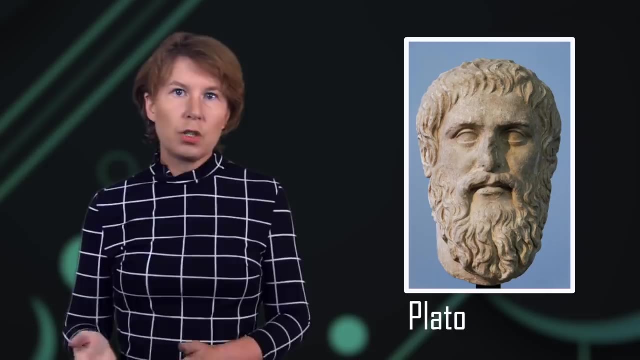 more. It's therefore possible that reality actually is math, But there is no distinction between them. This idea is not in conflict with any observation. The origin of this idea goes all the way back to Plato, which is why it's often called Platonism, though Plato thought that the ideal mathematical forms are somehow beyond human. 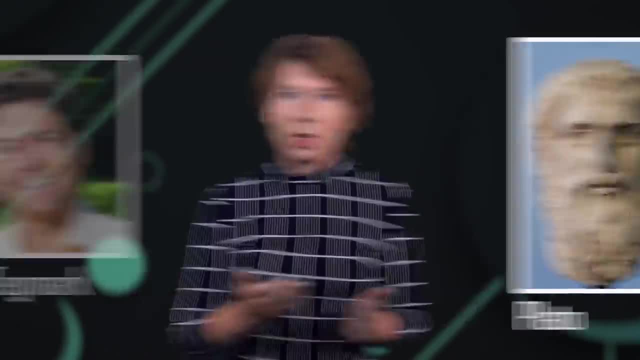 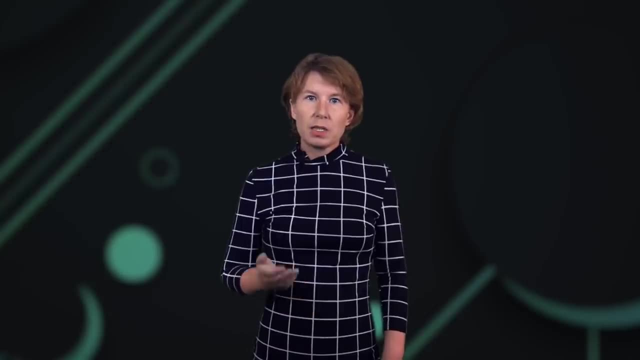 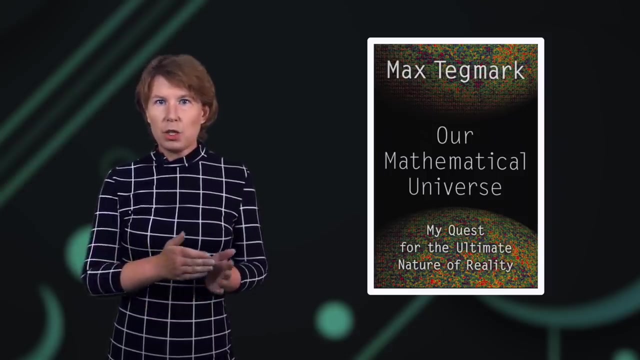 recognition. The idea has more recently been given modern formulation by Max Tegmark, who called it the mathematical universe hypothesis. Tegmark's hypothesis is actually more than that. He doesn't just claim that actually reality is math, but that all math is real. 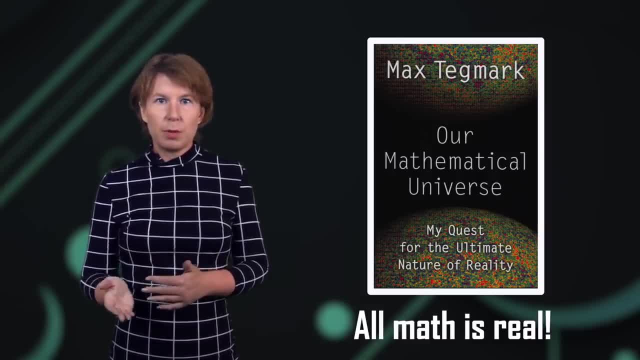 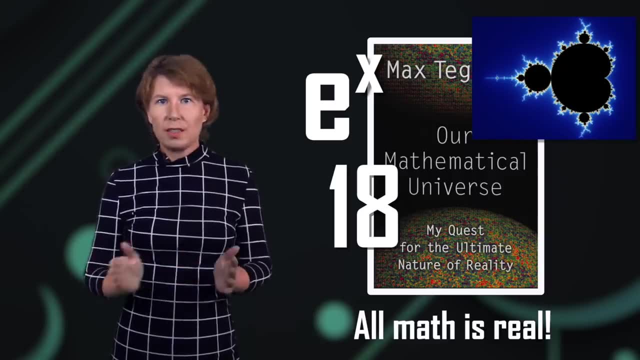 Not just the math that we use in our theories that describes our observations, but all of it. The exponential function Mandelbrot sets the number 18, it's all as real as you and I If you believe Tegmark. But should you believe? 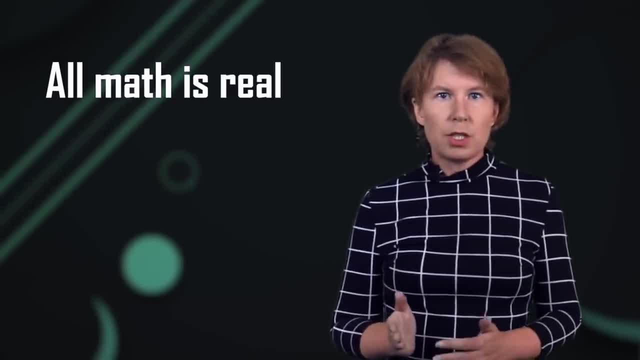 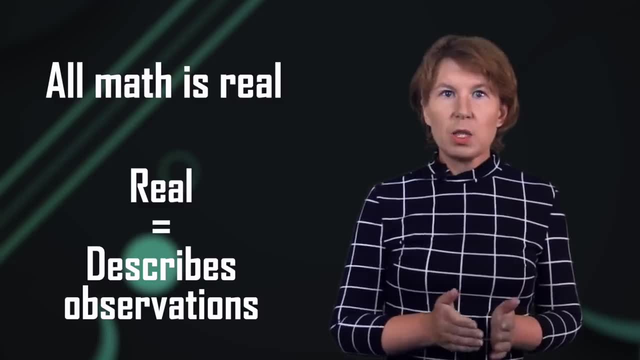 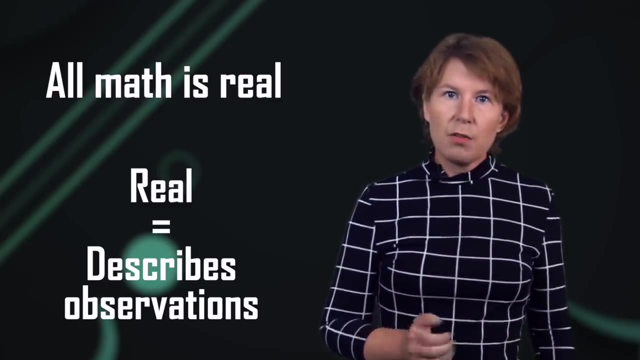 Tegmark. Well, as we have seen earlier, the justification that we have for calling some mathematical structures real is that they describe what we observe. This means we have no rationale for talking about the reality of mathematics that does not describe what we observe. Therefore, the mathematical universe hypothesis isn't scientific. This is generally. the case for all types of the multiverse. The physicists who believe in this argue that unobservable universes are real because they are in their math. But just because you have math for something else doesn't mean that they are real If you believe in something. 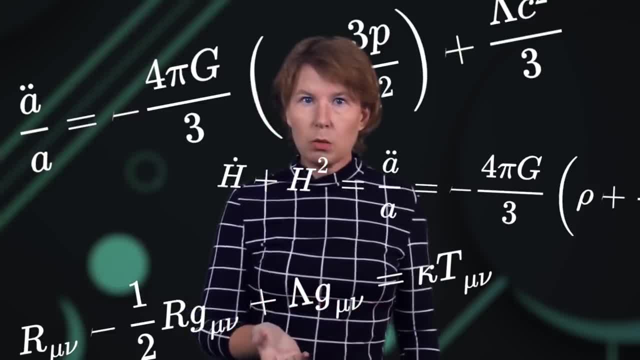 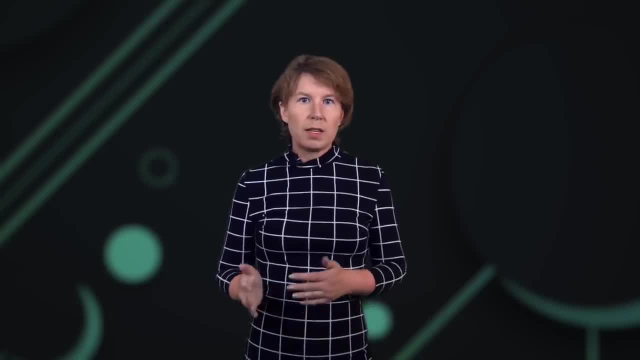 it doesn't mean it's real. You can just assume it's real, but this is unnecessary to describe what we observe and therefore unscientific. Let me be clear that this doesn't mean it's wrong. It isn't wrong to say the exponential.